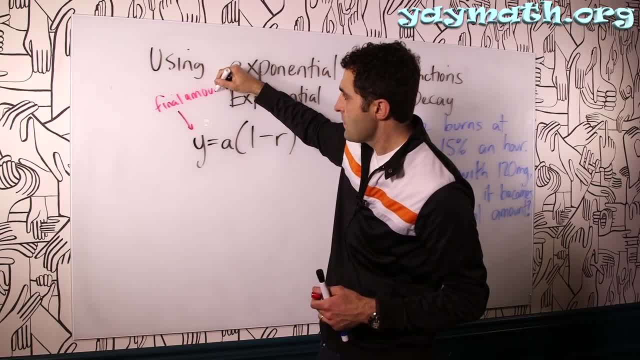 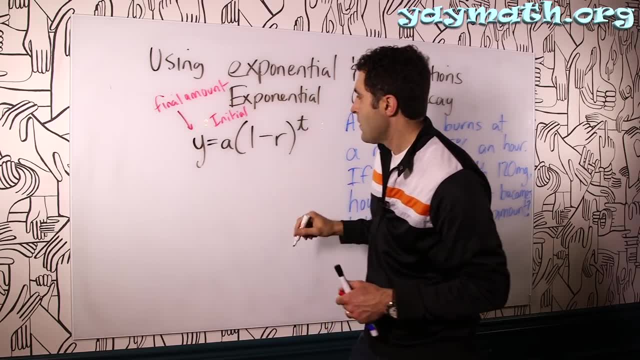 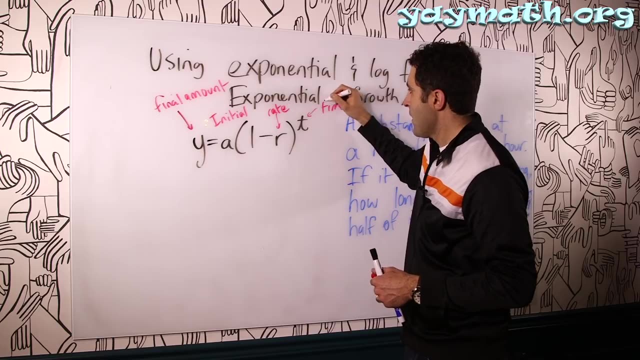 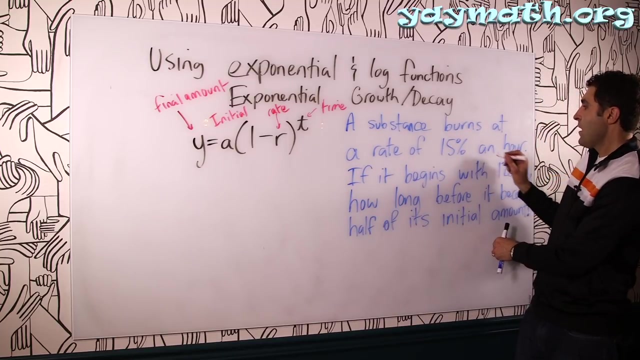 the one we're solving for the final amount. This a. this is the initial amount. Rate is r here And this is increments of time, And that time can be based on the problem specifically sometimes years. In this case, it looks like the increments of time is every hour. 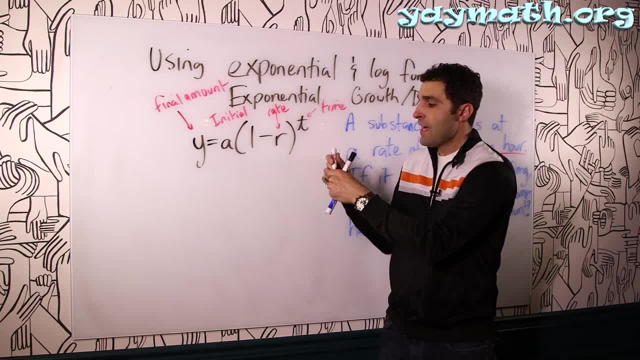 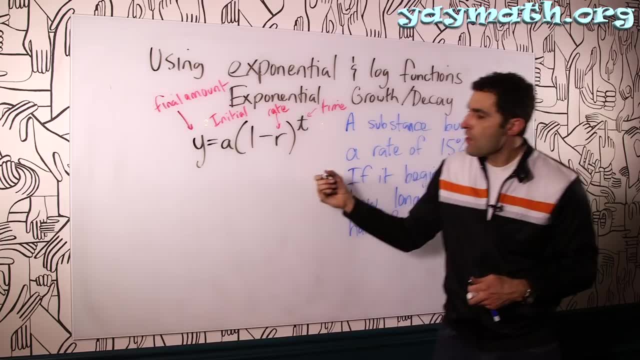 So we plug in everything that we need, or everything we know, into the formula and calculate what we need. So let's go ahead and discover how much is left. So we know, for example, the starting amount is 120.. That's going to go here. 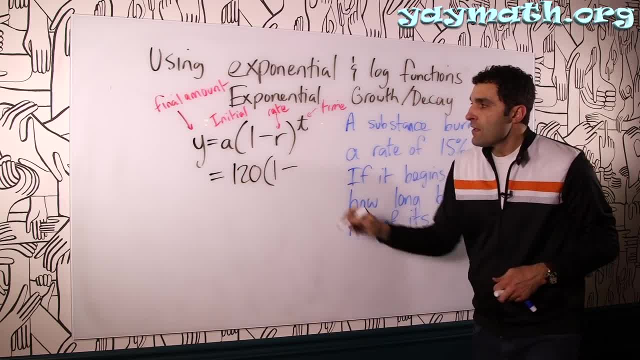 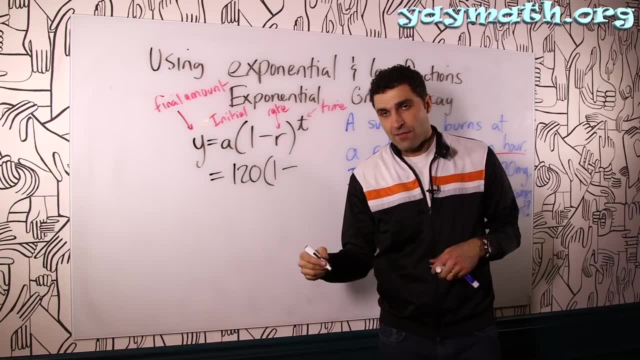 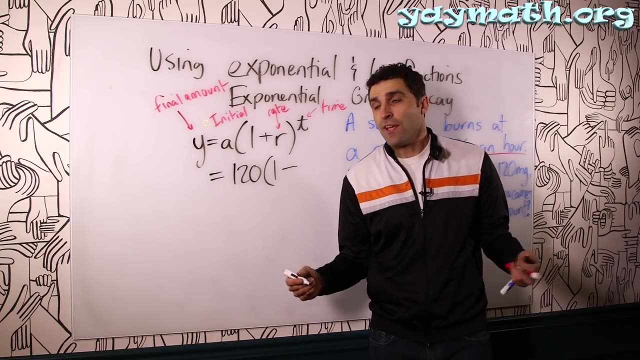 One minus. The reason it's minus is that this particular problem is a decay problem. The substance is going down. Had the rate been positive, like plus here, that would be something like if a population is growing or even money in a bank account is growing. 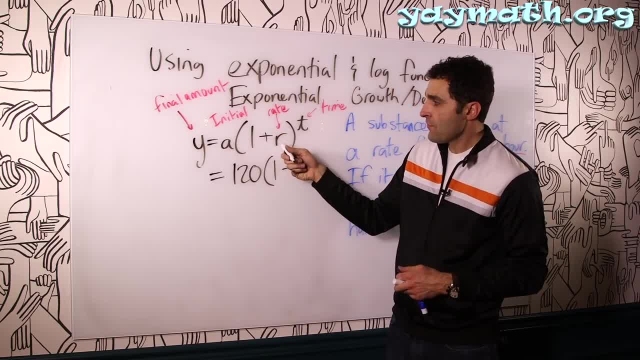 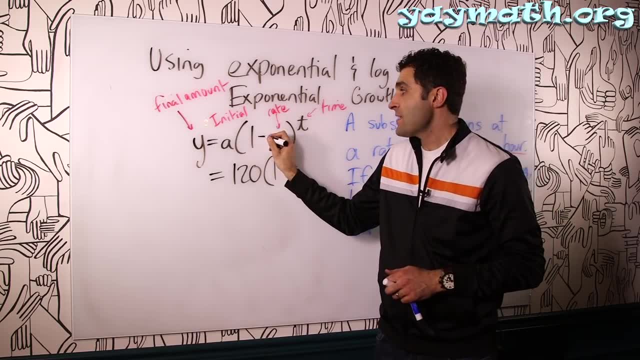 with interest over time. that would be adding the rate, whatever that percentage is, to one, which would represent the 100% that you're adding to. But in this case we're subtracting because we read into the problem and the substance. 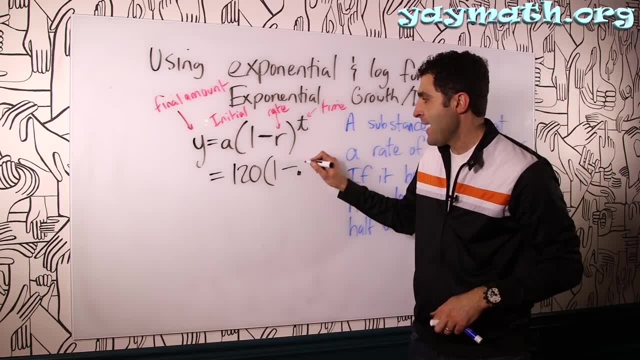 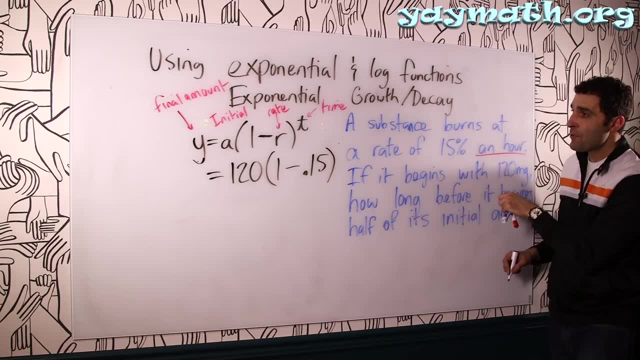 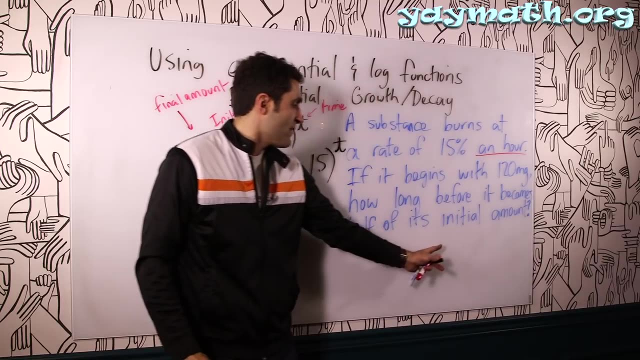 is burning, It's burning down, So it's actually decaying, It's decreasing in its amount And we're actually looking for the amount of time it would take- which t we don't know- for the 120 to become half of its initial amount, Half of its initial amount, So that 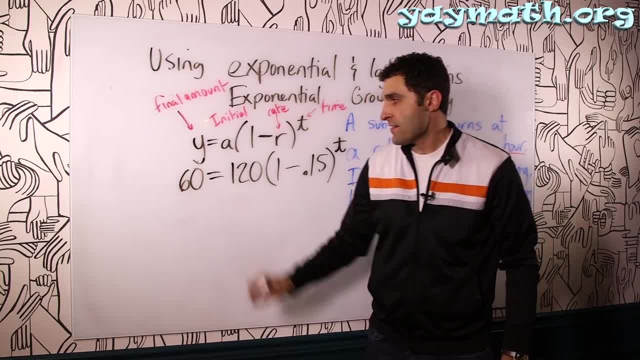 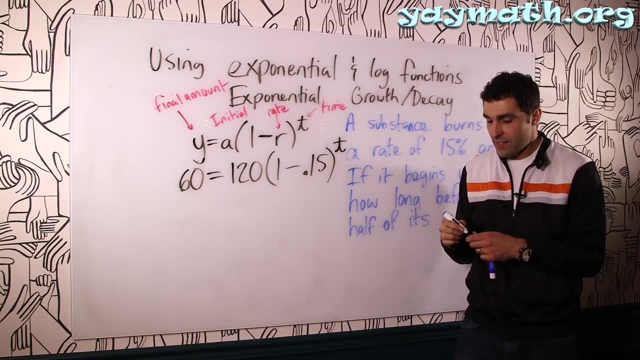 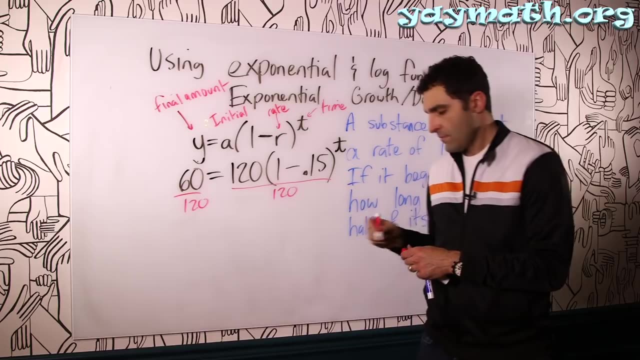 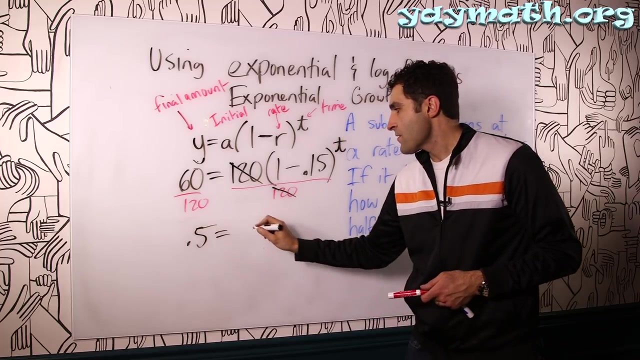 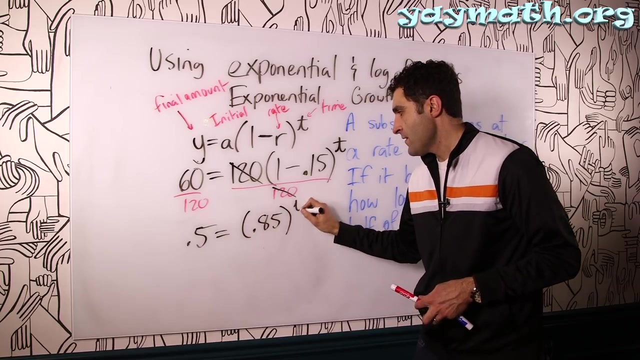 would mean the 120 needs to reduce to 60. And now we have a single variable in there, which is t in this case. So let's go ahead and solve. We can divide both sides by 120 to simplify our lives. There it goes. So this is 0.5 equals 1 minus 0.15 is 0.85.. So that's 0.85 to the t. 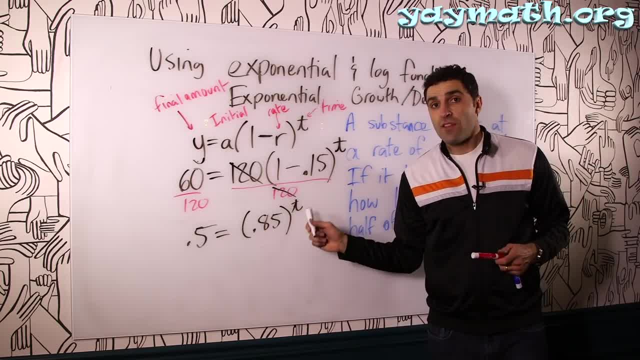 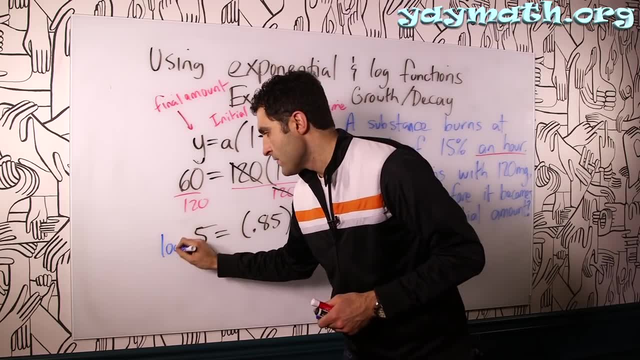 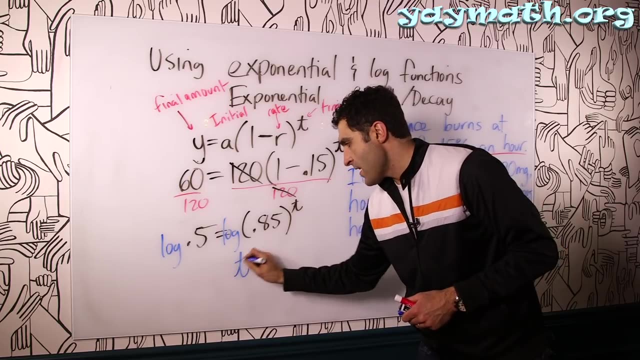 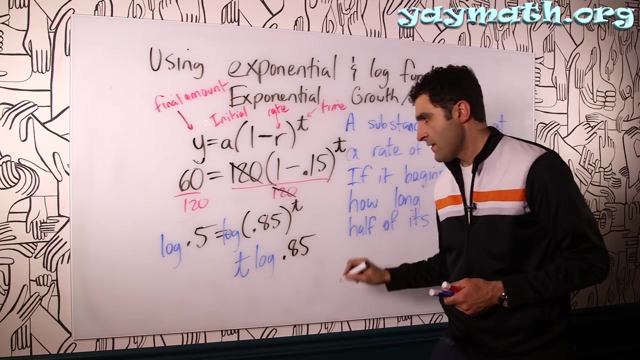 Okay, All right. The way to solve these is to use logs to our advantage. So if we take the log of both sides- log here and log here- this t can move down in front of the log, So that becomes t times log of 0.85.. And this is log of 0.5 equals. And if we want to get t, 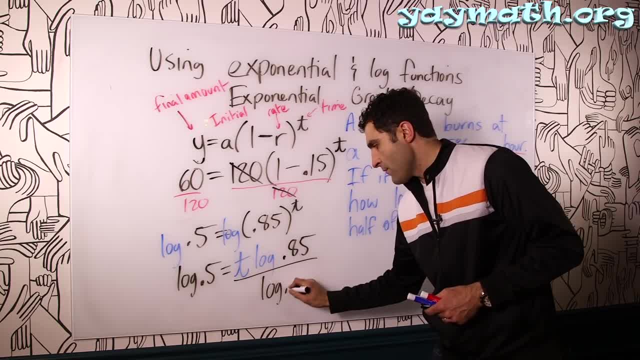 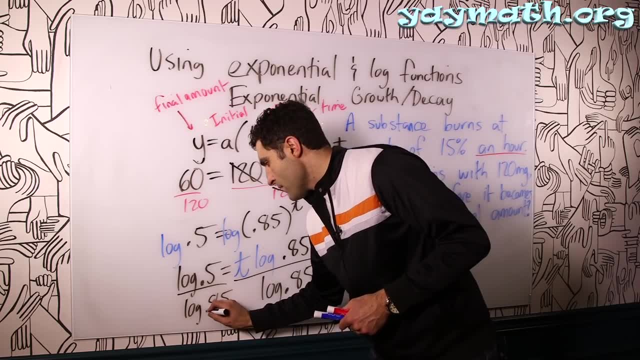 by itself. we're going to have to do this. So we're going to take the log of 0.85 and we're going to divide both sides by log of 0.85.. Log of 0.85.. And we should get our. 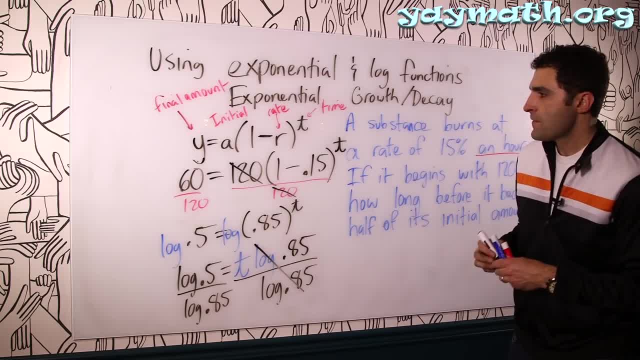 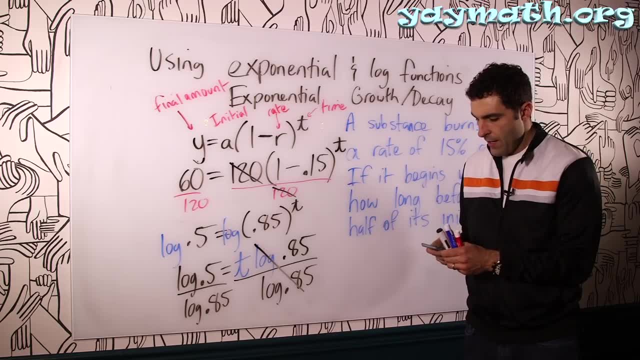 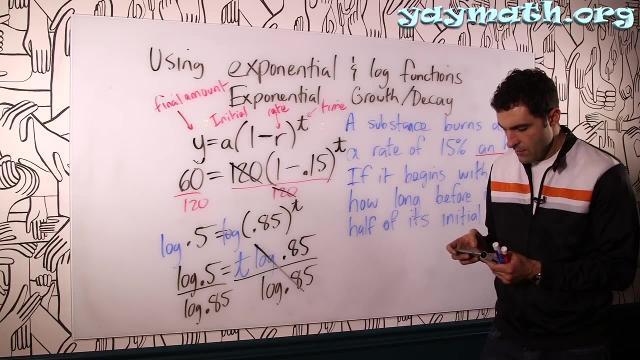 answer And this would go: Let's see what happens. Handy dandy, calc, There we go. Okay, We'll do 0.5. log of 0.85.. Okay, Okay, 1 plus divided by: And 1 plus divided by: 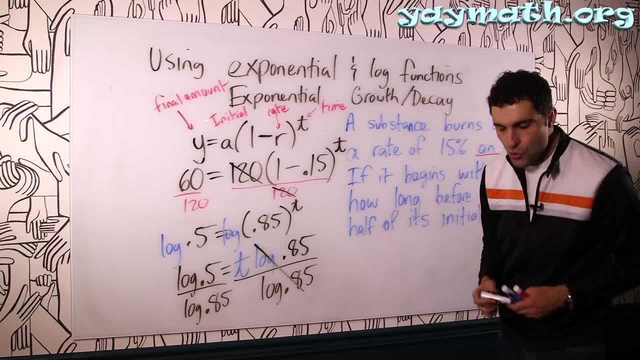 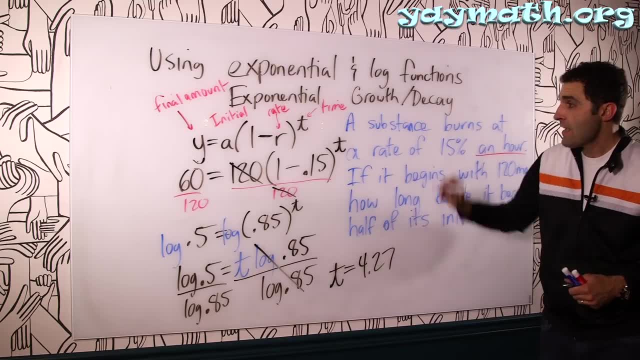 divided by 0.85, log equals 4.27.. Time equals 4.27. In this case, hours, Okay, And it makes sense. In one hour it goes down 15% of itself. Right Another hour, 15% of. 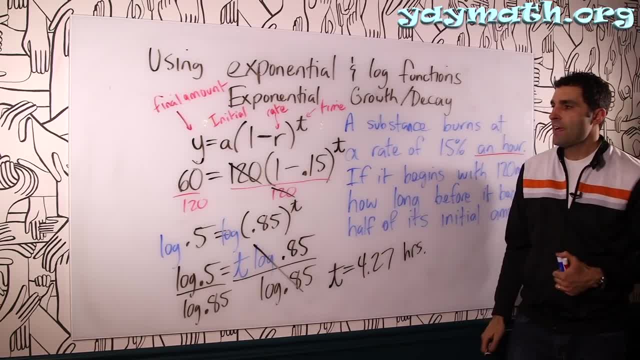 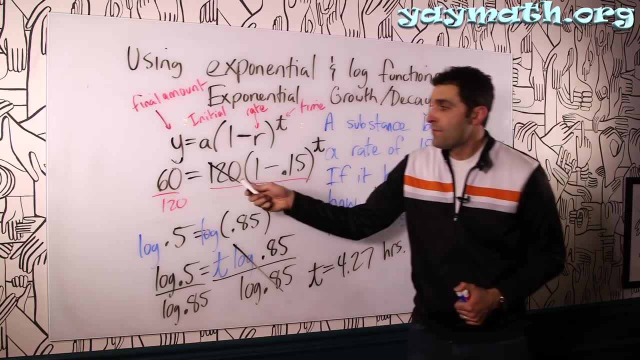 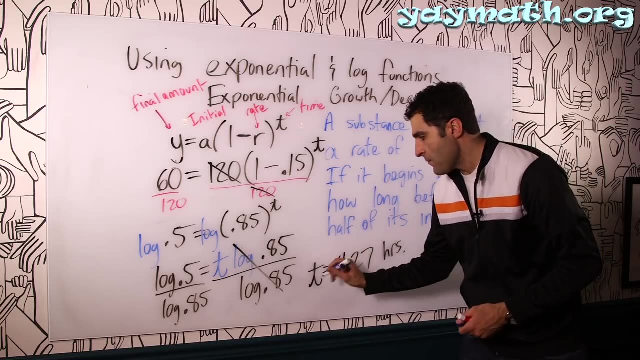 that Now the hour, 15% of that. After four hours it probably goes down 15% in its process. All right, Let's say you have all four staff. Okay, Yes, probably went down 50% from 120 to 60. This amount of time right here is a very 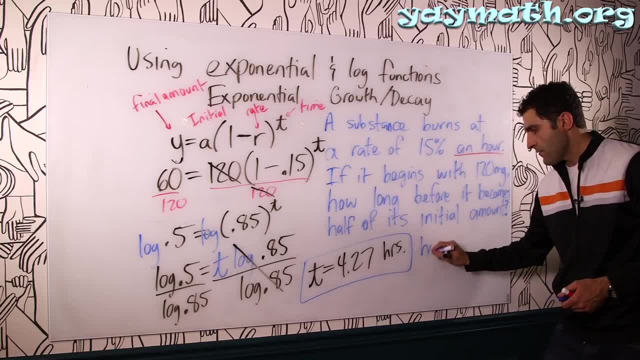 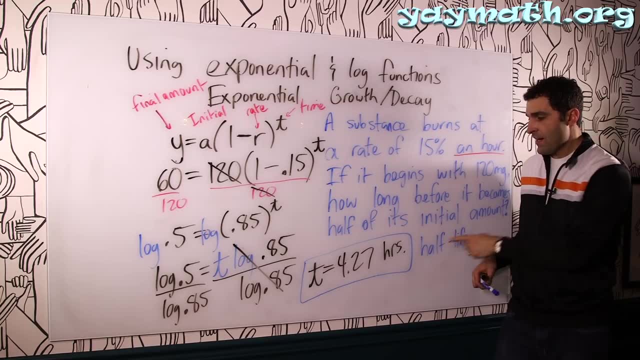 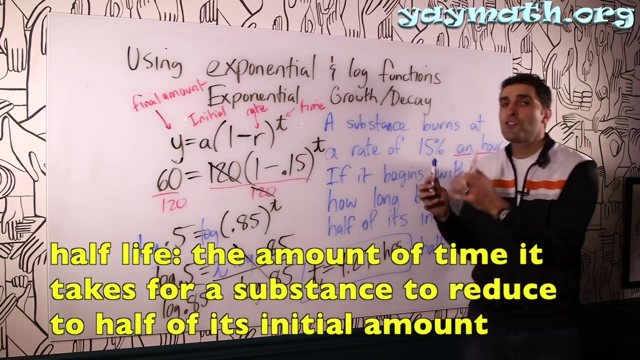 important increment. This is called half-life. Let's define that right now because it's going to feed into the next problem. The next problem talks about half-life. Half-life is the amount of time it takes for a substance to reduce to half of its initial amount. Again, half-life is a measure of time. It's the 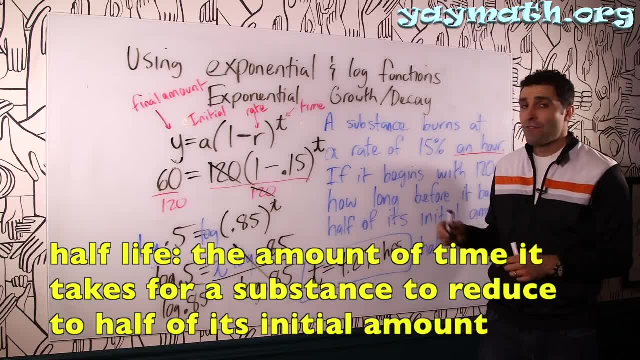 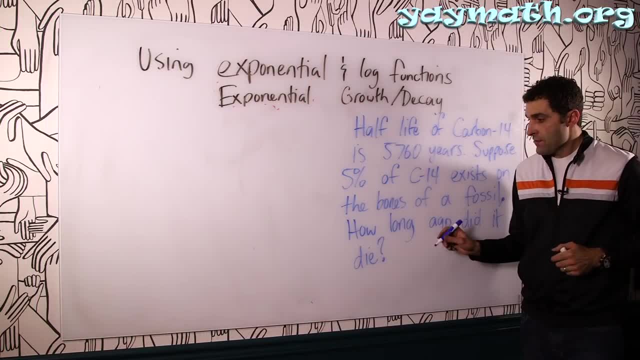 amount of time it takes for a substance to reduce to half of its initial amount. Okay, great. So this next problem is a half-life problem and we're going to use it to backdate fossils. Let's first present the problem, The half-life. 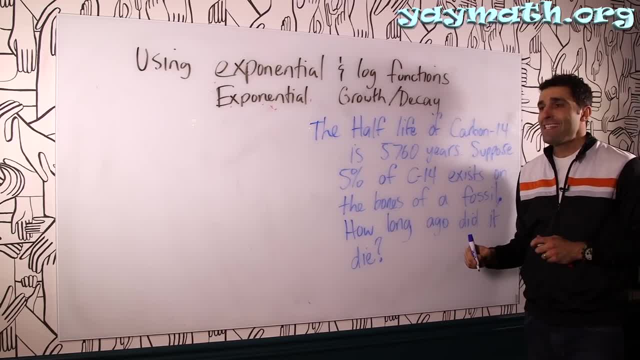 of carbon-14 is 5,700.. Let's first present the problem. The half-life of carbon-14 is 5,700.. Let's first present the problem. The half-life of carbon-14 is 5,700. It's 5,700 years. Suppose 5% of carbon-14 exists on the. 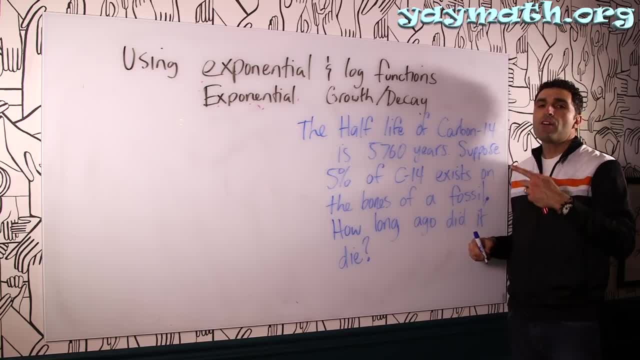 bones of a fossil that was discovered Five percent of what we expected- the expected amount of carbon-14, in what would otherwise be an alive creature. Maybe it was some dinosaur, a saber-toothed tiger or something like that, But we see, we observe 5% of carbon-14 within the bones of this fossil. 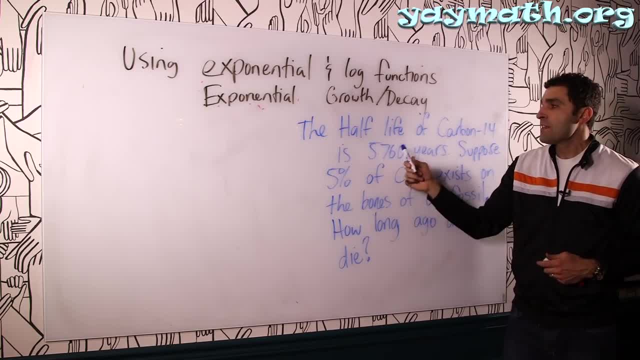 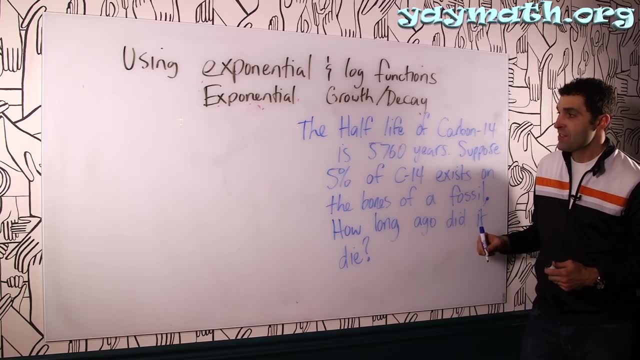 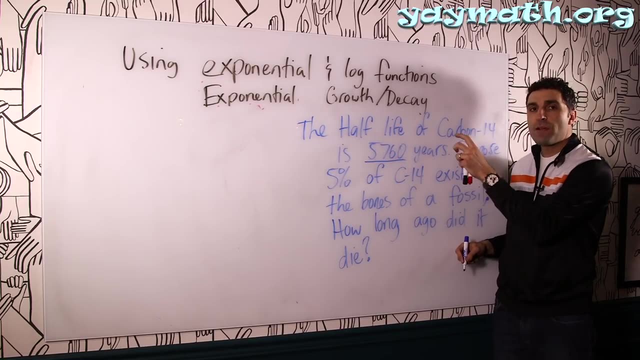 If there's five percent left, knowing that the half-life of carbon-14 is 5,700, 760 years, how long ago did this particular animal pass on? This is kind of amazing. right Again, let's discuss what half-life means. This is the amount of time it takes for a substance to go. 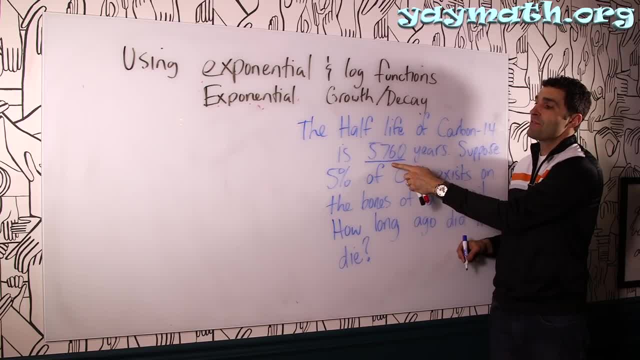 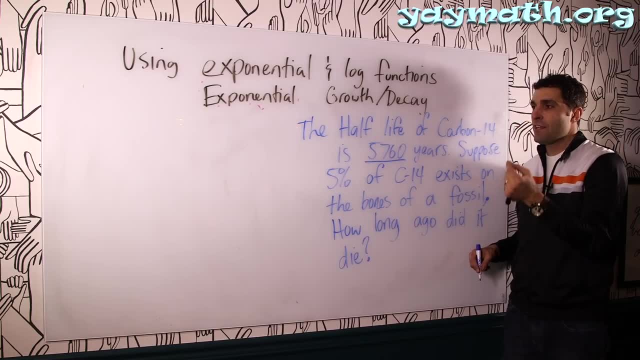 to half of its original amount, You'll notice it's a lot of time. So carbon-14 is an element that sort of dies off that disintegrates very slowly. Therefore, we can use that to backdate fossils for when they're actually living and breathing. So what we need to do is we need to understand. 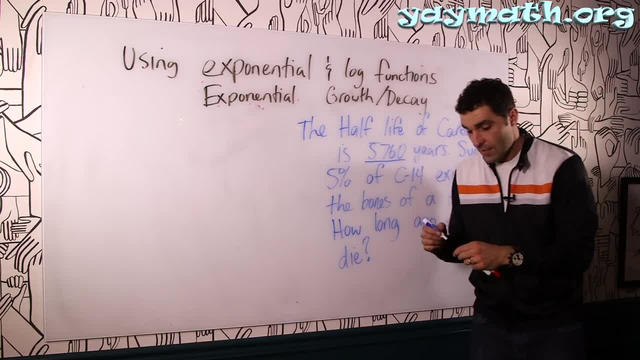 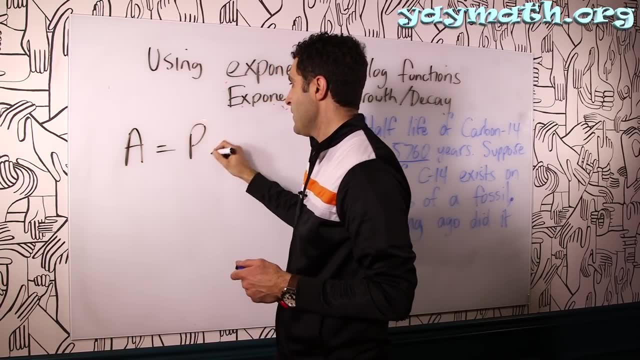 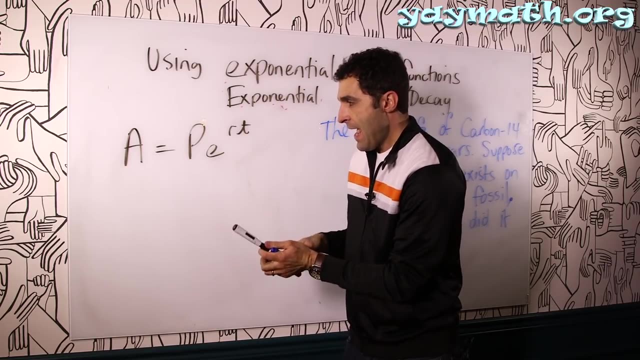 the rate of decay of this particular fossil. Let's introduce the formula for that. Students call it Apert. A equals P-E-R-T. This is just like the formula from before. You'll notice this end amount here. this is the final amount. This is the final amount. 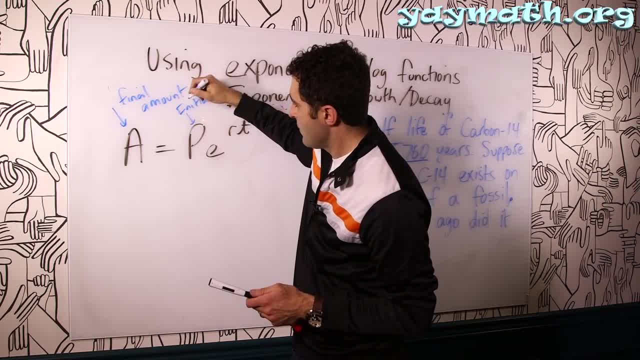 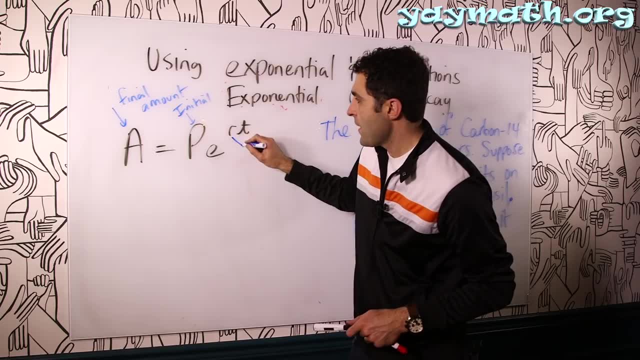 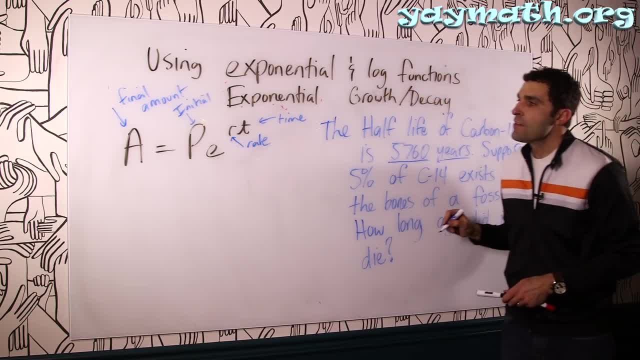 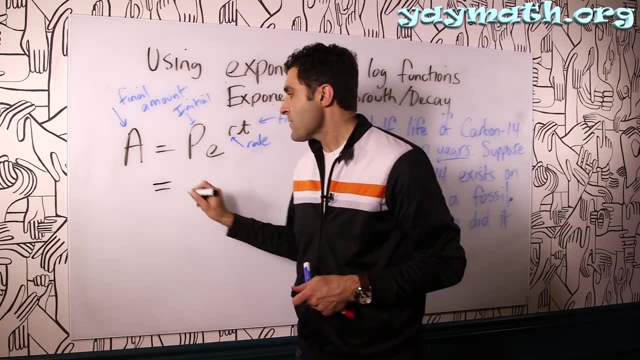 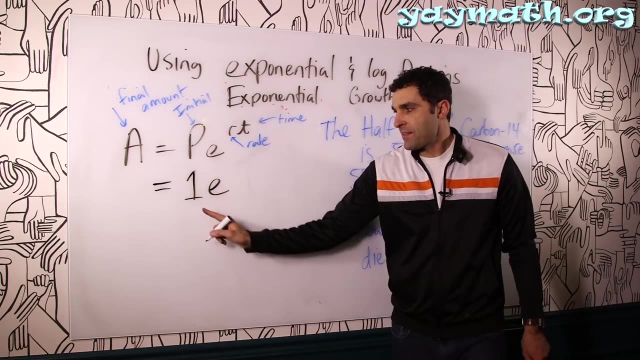 measured in years. All right, so what we're going to do first is we're going to find the rate of decay of this fossil. Let's do it If something starts at one unit, hypothetically, you know. just to make it simple, we have E, the rate. we don't know. 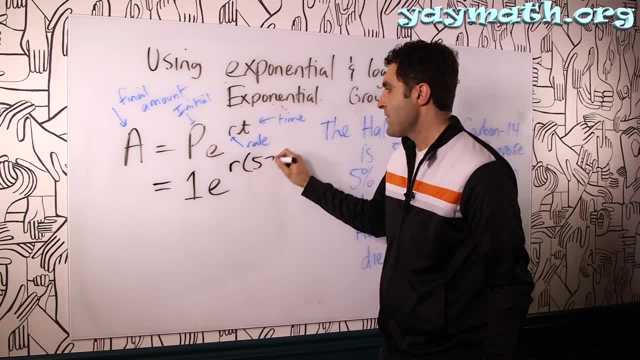 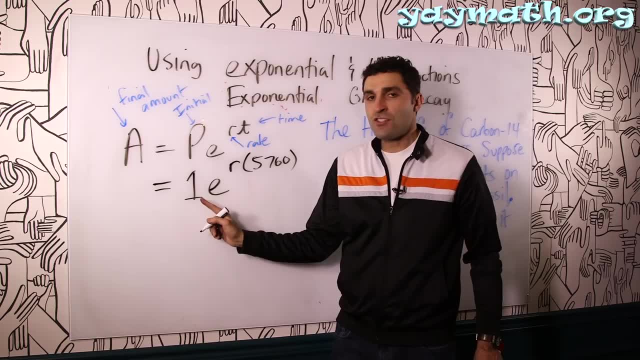 the rate of decay. The time in this case is 5,, 7, 6, 0.. And it takes 5,, 7, 6, 0 years to go from one, an initial amount of one, to half of itself. That's what half-life is. 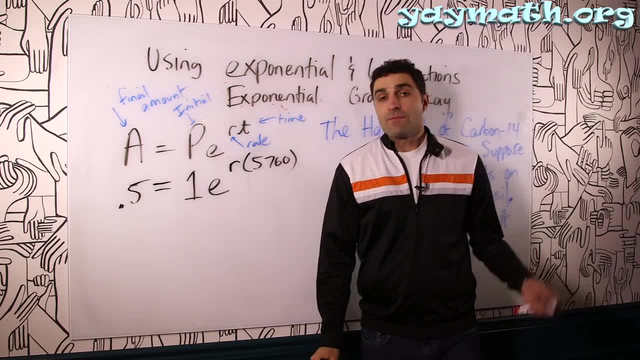 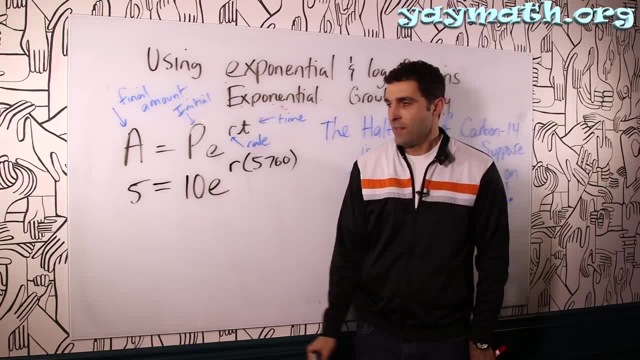 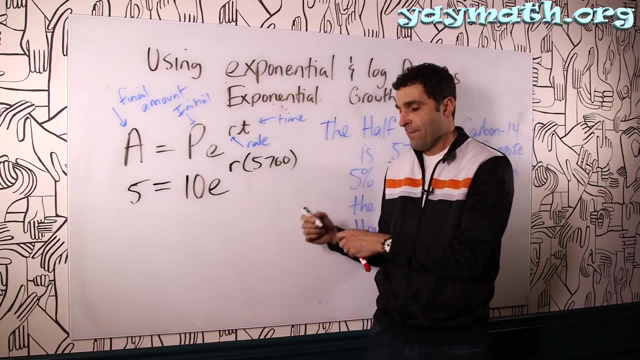 you would end with 5.. It's totally fine to put it that way: Start with 10, end with 5.. It takes 5,760 years, And then we're going to solve for the rate of decay. All right, here's how we do it. 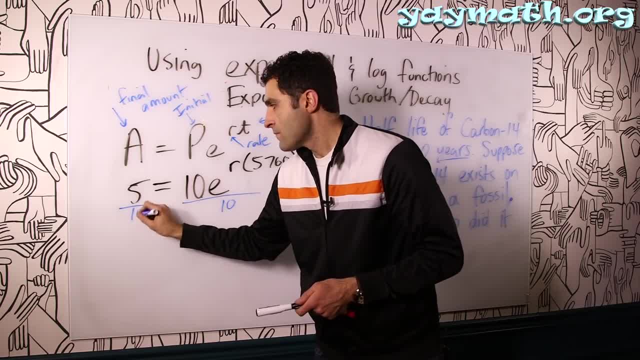 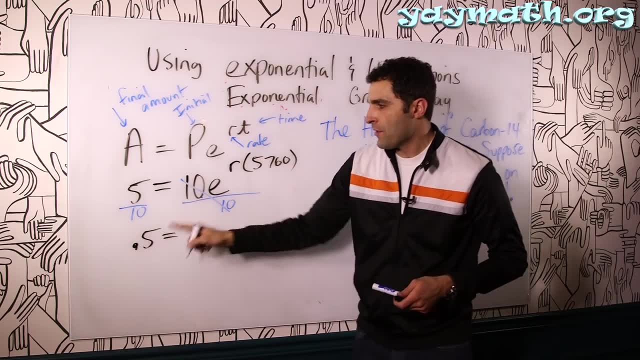 Divide both sides by 10.. Gone 5 over 10 is 0.5, which is exactly what we wrote before, when I had 0.5 and 1.. This was 1 here. E to the 5,, 7,, 6,, 0.. 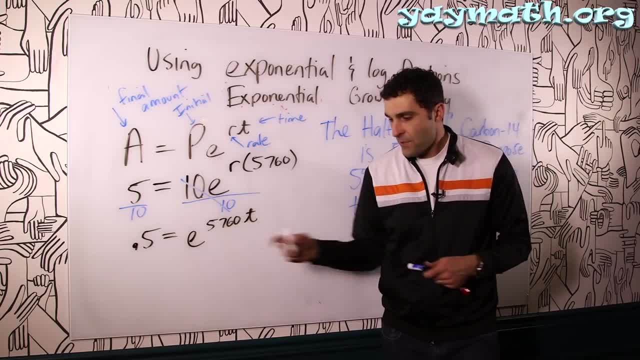 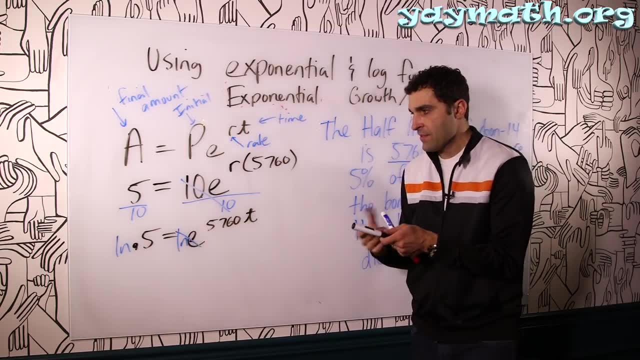 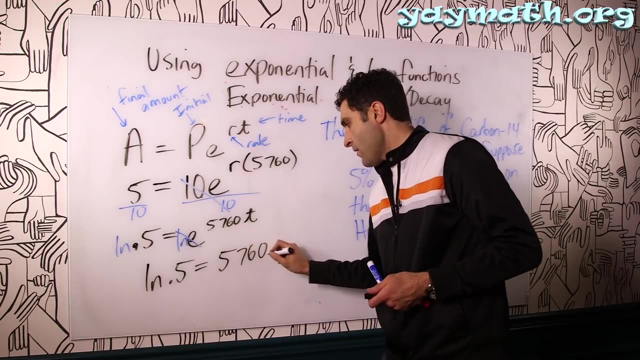 Yep, T. And if we want to cancel this E, we do LN of both sides. This is LN here, LN here. This is gone. LN and E cancel each other. We have LN.5 equals 5, 7, 6, 0, T. Divide both sides by 5, 7, 6, 0.. 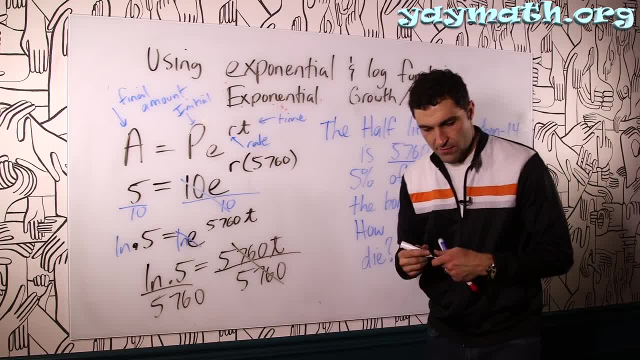 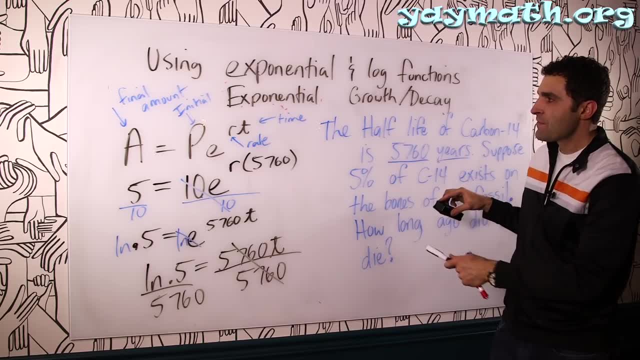 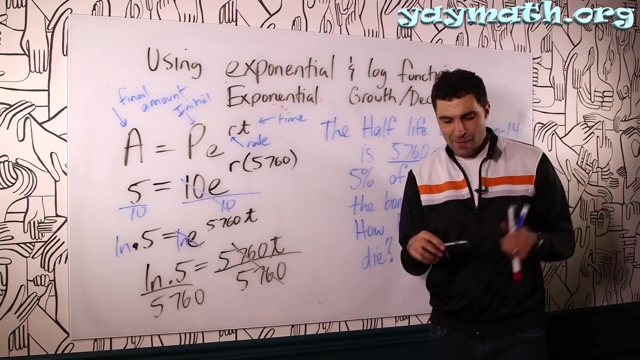 5, 7,, 6, 0. Gone, Yay, math. I don't want to mess up the problem so I'm going to put it over. Actually, I can solve on the calculator. That's just people walking by and looking through the glass trying to get their. 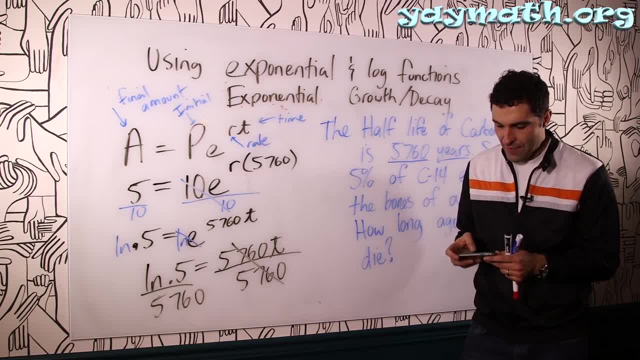 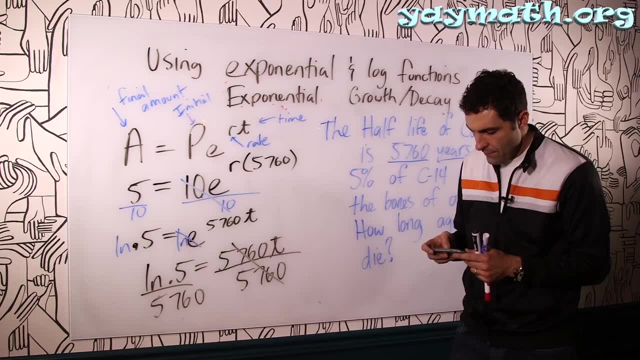 education on. All right. so we got 0.5 LN. It's kind of cool. We're doing all these high-level calculations right on the phone. Divided by 5, 7, 6, 0.. Yeah, There it is Negative 0.0,. 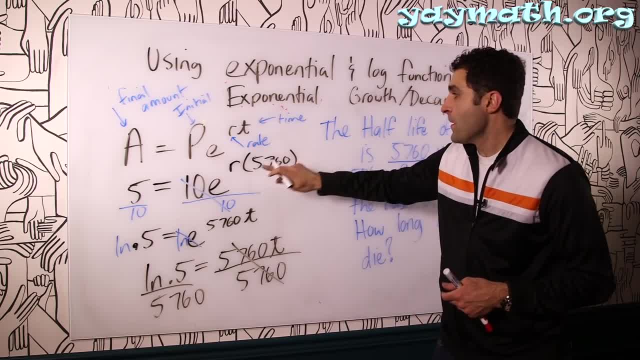 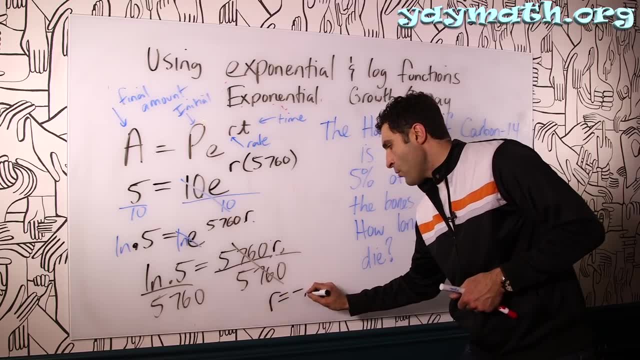 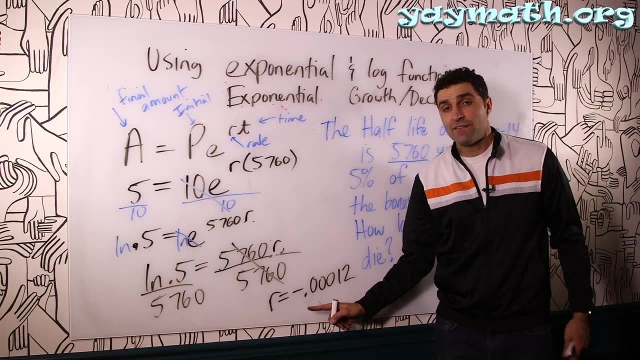 0,, 0,, 1, 2.. Oh, that's R. Excuse me, R It's the rate Solving for the rate. R equals negative: 0.0,. 0, 0, 1, 2.. So it's a very, very slow rate of decay. And notice, the rate is negative. 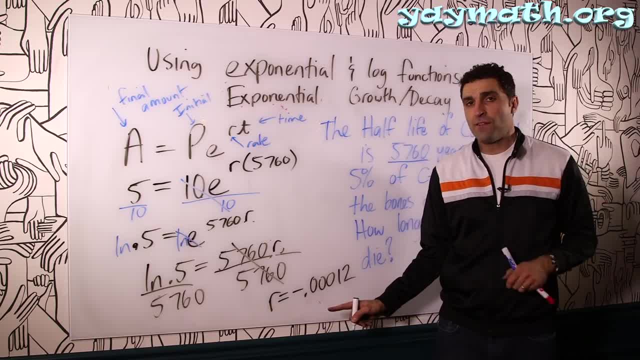 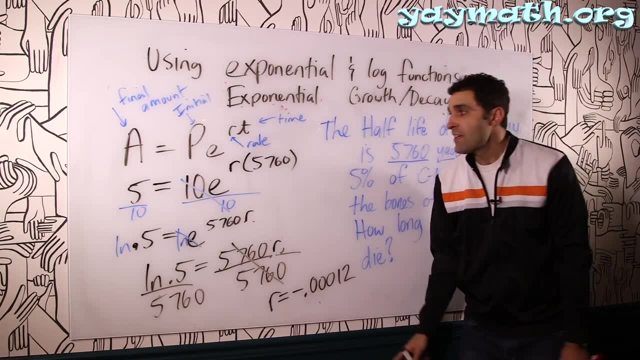 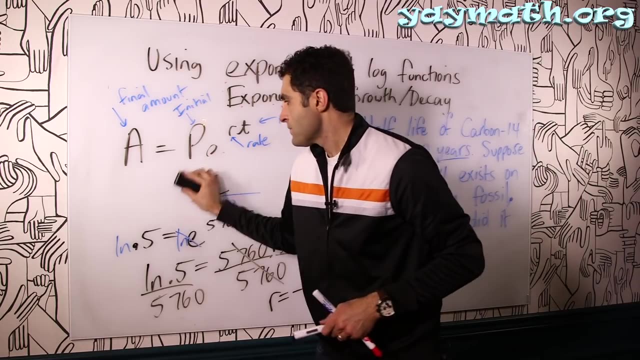 just like the one where the element was burning off at 15%. So that rate was negative. So, too, this rate is also negative. So we're going to use this rate to backdate the fossil That has 5% carbon-14 left. We use the same formula again. We use the same one. We'll use. 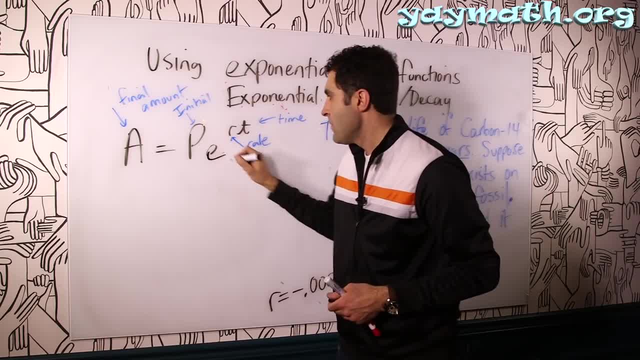 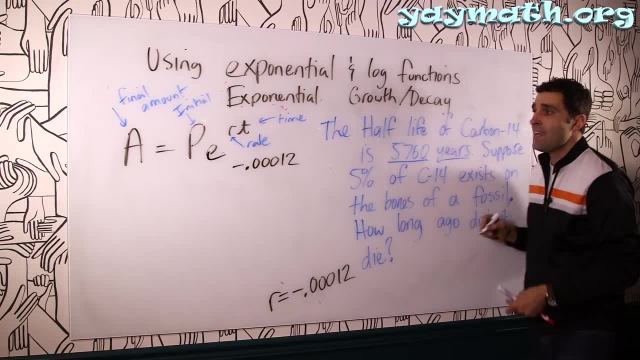 that same rate. So in the problem we could do a rate of negative: 0.0,, 0,, 0,, 1,, 2.. And the problem's saying: how long ago did it die, How long did it take? So that's a T We. 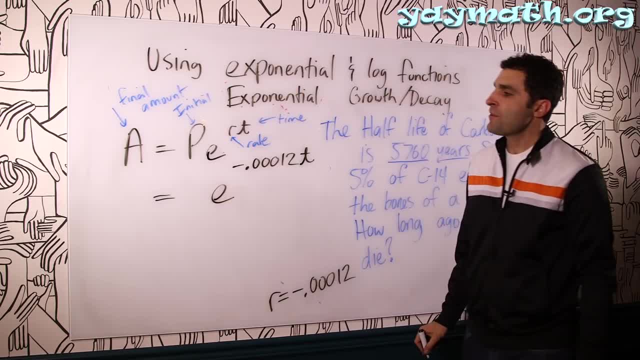 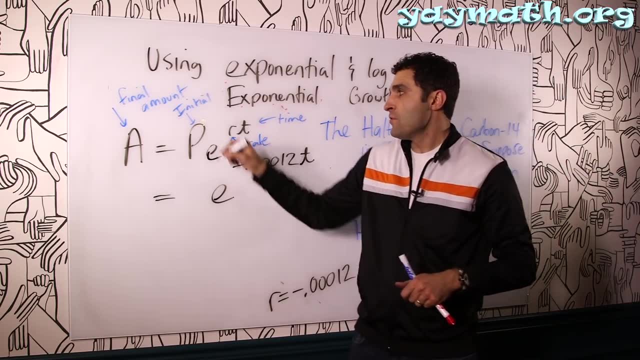 don't know E. And now the challenging part of the problem: 5% is left. 5% is left, No more. And so, knowing what we know about percents, we can assume, just as an easy example, 100. 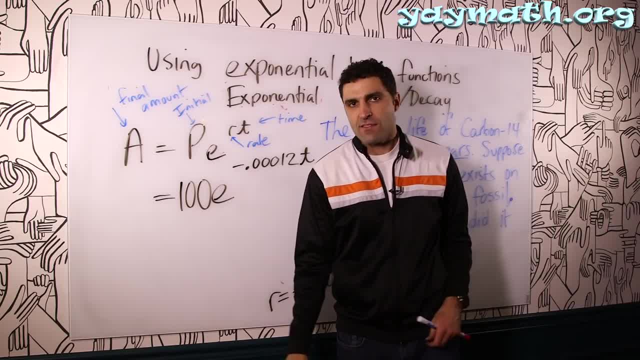 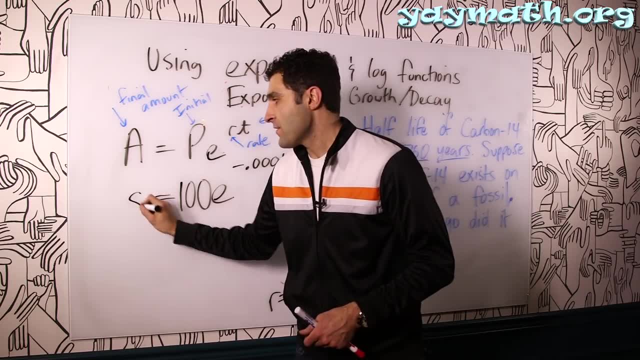 could be a starting amount. So imagine it had 100 grams to start some sort of random amount- It won't matter- And the final amount is 5% of that. 5% of 100 is 5.. So this would 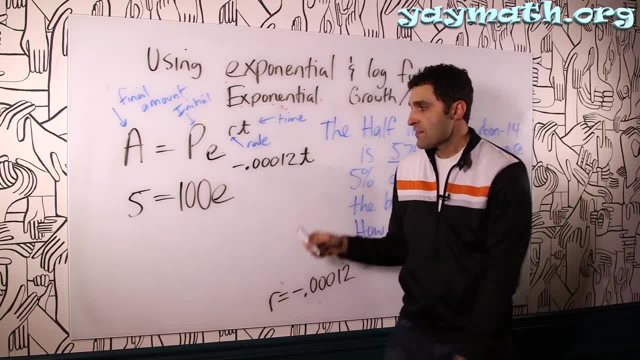 be the setup to solve for the amount of time it takes to go from 100 units of carbon-14 to 5 units of carbon-14.. 1.0. 2.0. 1.0. 1.0.. 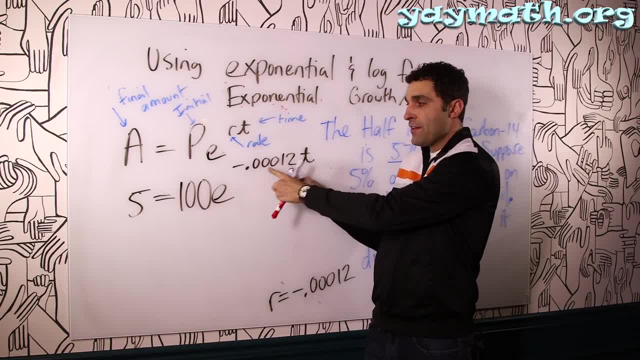 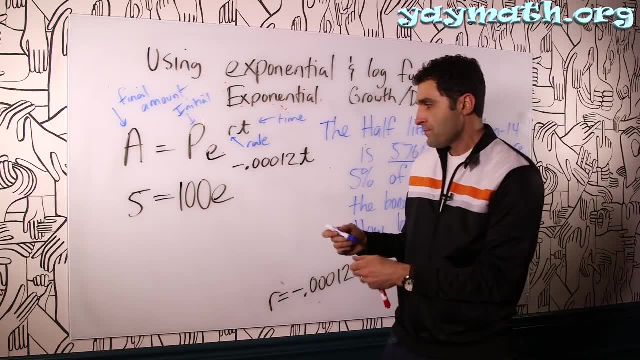 1.0.. This ridiculously slow rate. It's a very small small number And it's negative, meaning it's decaying, It's getting smaller. And now we solve for T Five, both sides by 100.. Five. 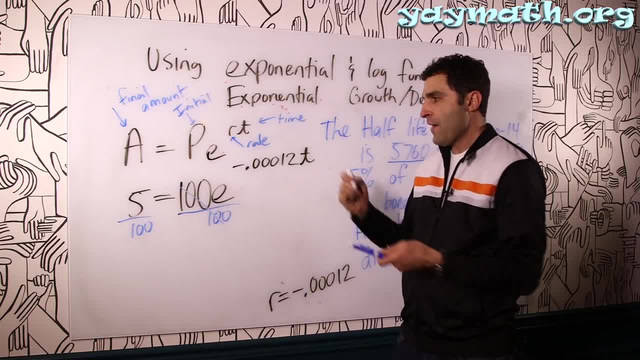 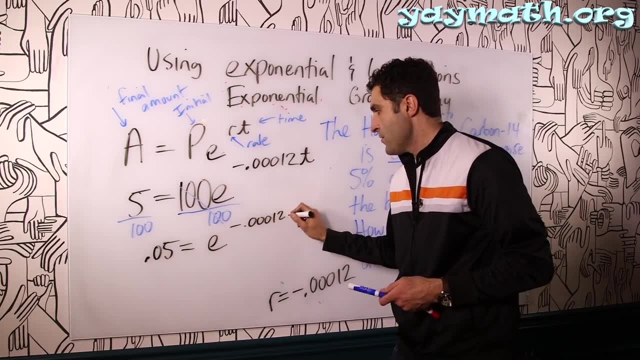 both sides by 100.. We're gone. We get that 0.05, which makes sense. We're talking about 5% Equals E to the negative 0.00012T. I'm so excited to be able to help you learn this. 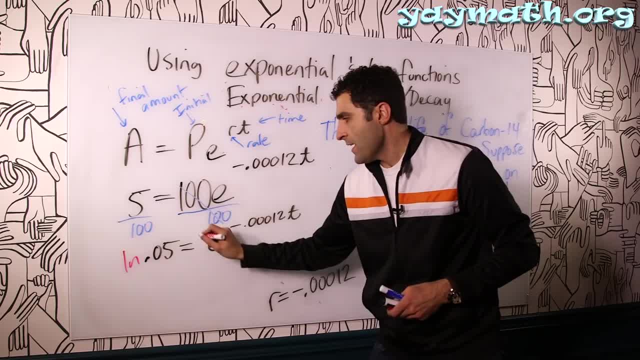 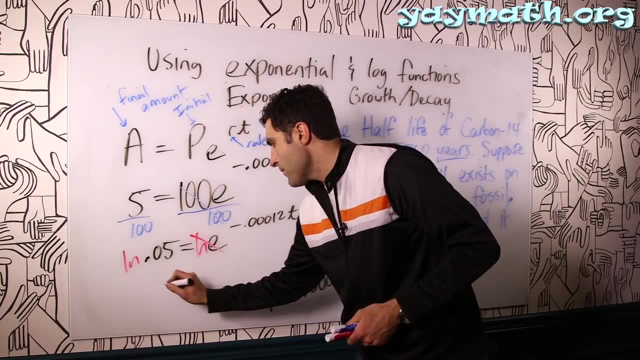 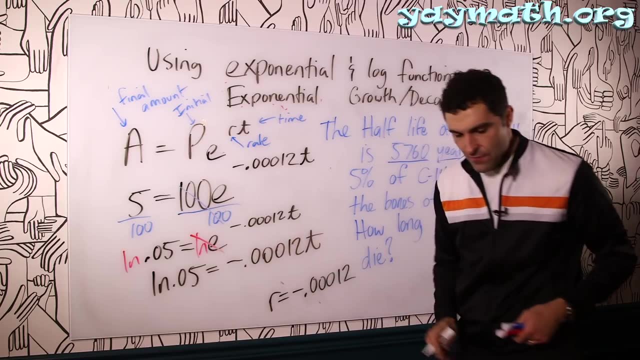 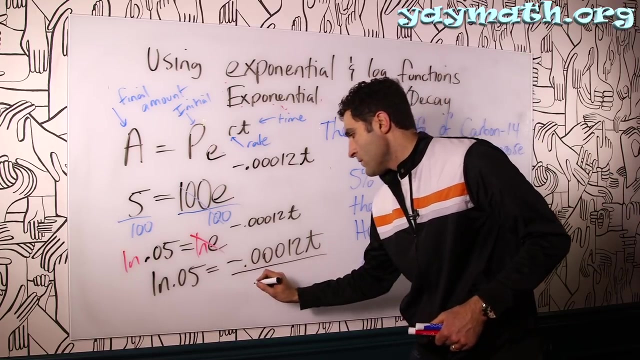 stuff, because it's really challenging if it's not explained appropriately. LN- both sides gone, We get LN.05 equals negative .00012T. Divide both sides by negative: .00012T- Negative. let's write it out, man. Let's write. 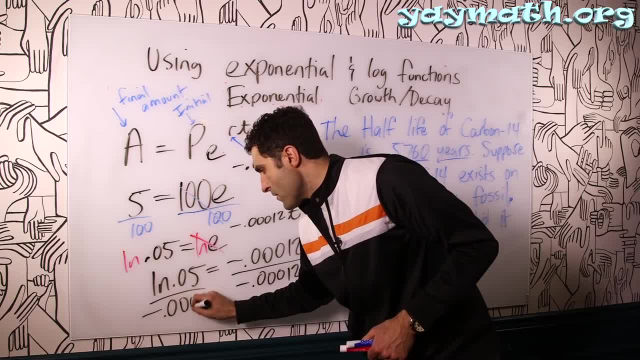 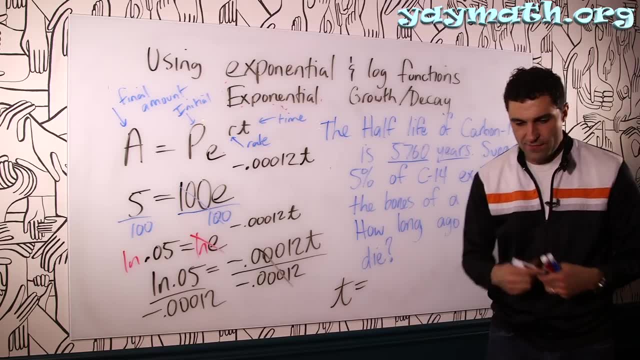 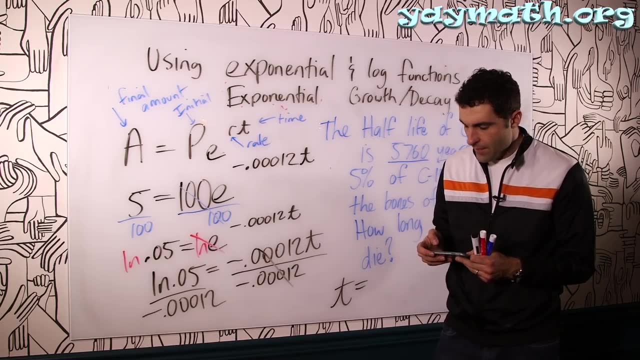 it out. Don't cut corners, baby. Negative: .00012, gone And we get time equals, all right. I'm curious, Find out what it is. Here we go: .05, LN divided by .00012, negative. 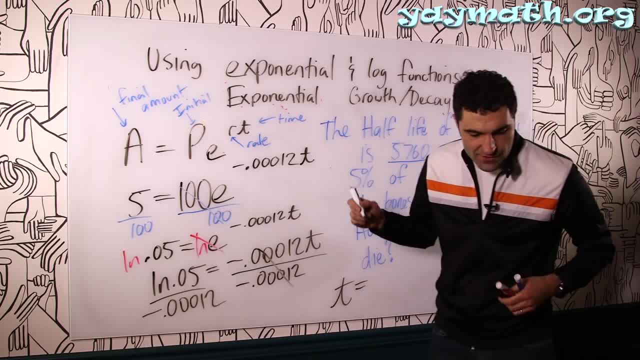 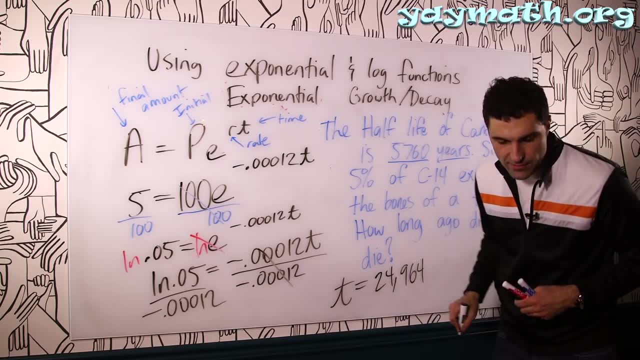 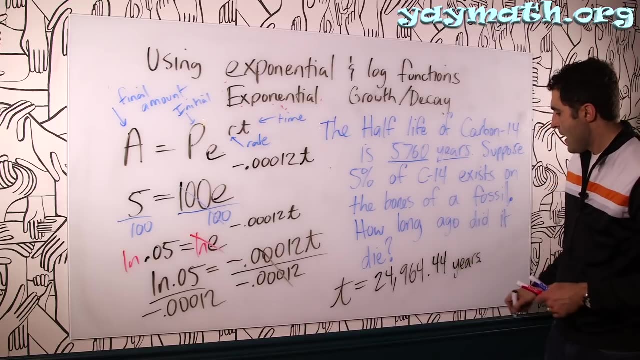 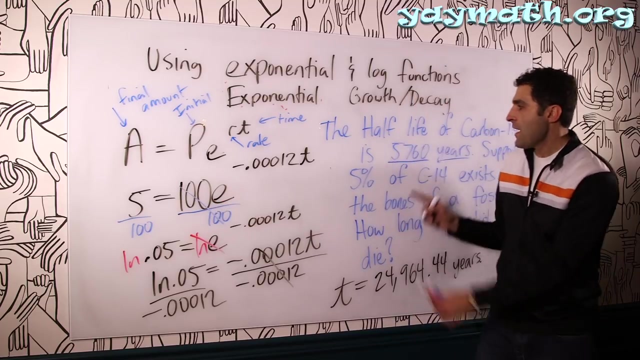 equals Wow, 24,964 T, .44 years. And pretty incredible how that works. And it makes sense if you think about it, because if it started at 100 and around 5,000, 6,000 years, it became 50. And then 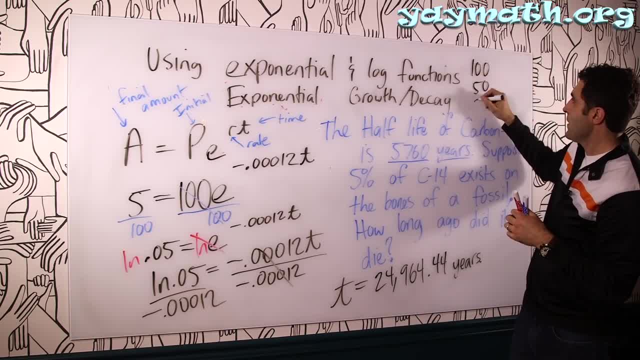 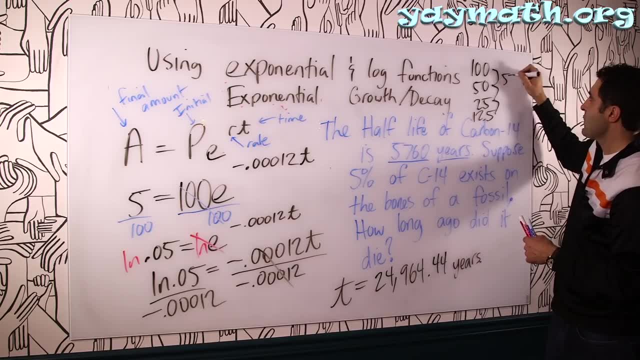 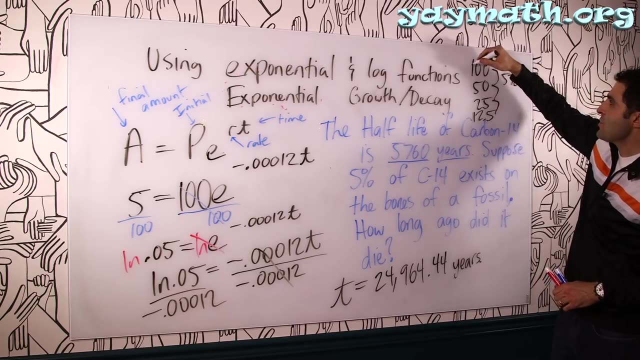 100, then it became 50, then it became 25, then it became 12.5.. You see where this is going. This cycle is 5,760 years, So you keep adding 5,760,, 5,760,, 5,760, and you keep slashing. 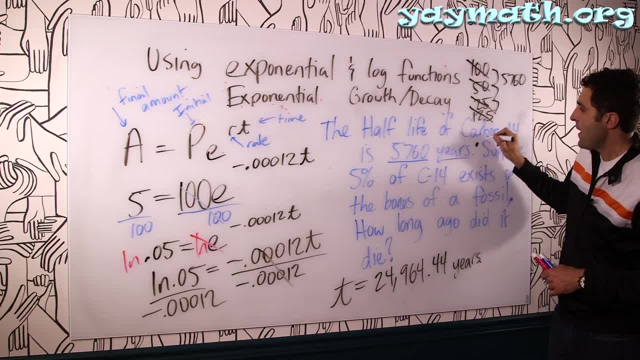 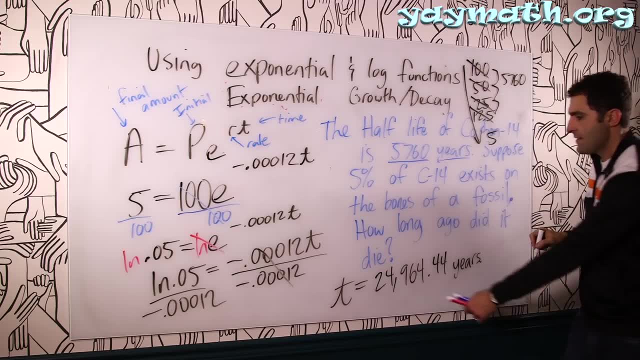 this in half, half, half half, until you get to .05, or 5%, or just basically 5.. 100 reduces to 5, and it takes this many years, which is about like what? five cycles of. 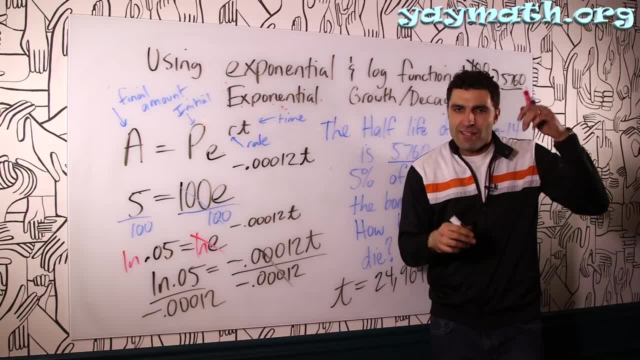 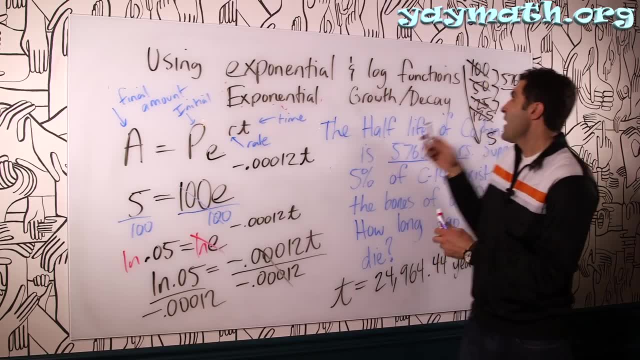 5,760 years. That's a good way to stay in command. It's a good way to stay in command of what's going on here, right? It starts at 100 and turns to 5,, so it's like half half, half half a certain number of times until you get. 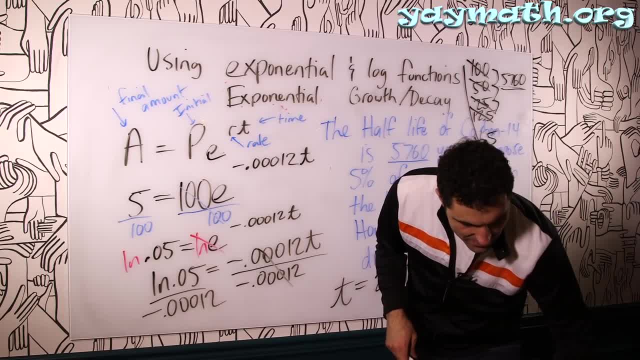 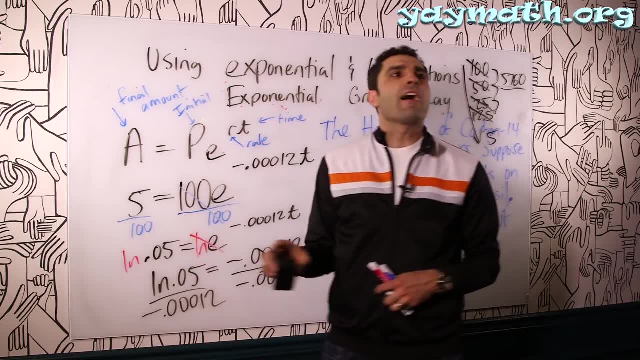 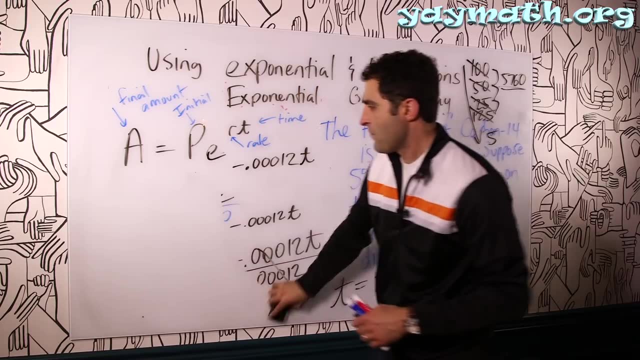 down to 5.. All right, We're going to do one more. I know this is a long one, but I'd rather just save it in one video, Or maybe not. What do you think? Yeah, just keeping it. Yeah, keeping it. yeah, Yeah. well, yeah, because then you're forcing. 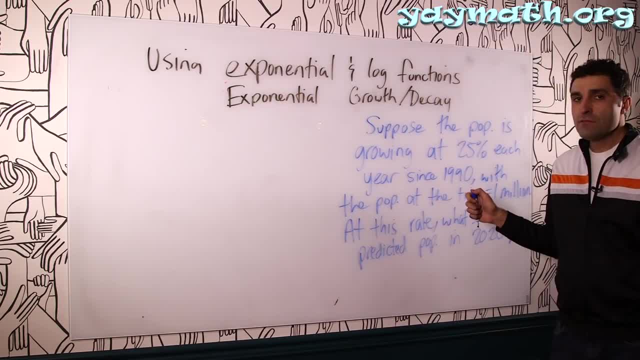 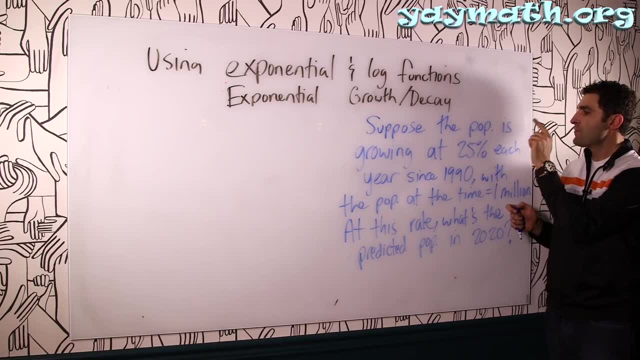 people to like remember the same thing. Then you're just like, Okay, cool. last problem, let's rock this. Here we have a population problem. Suppose the population is growing at a rate of 25% each year since 1990, with the population? 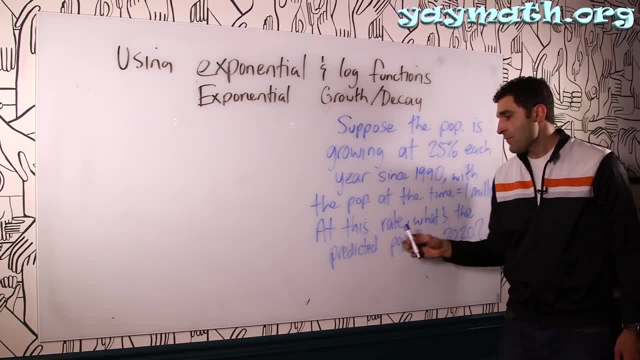 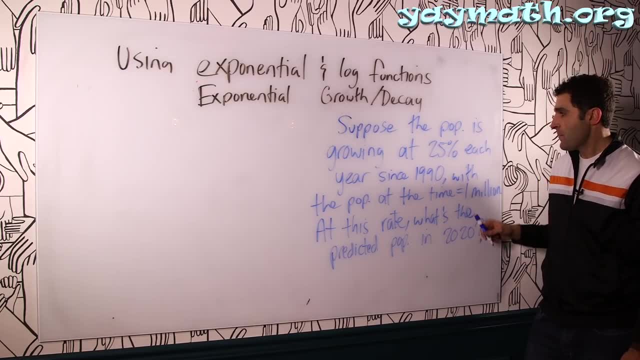 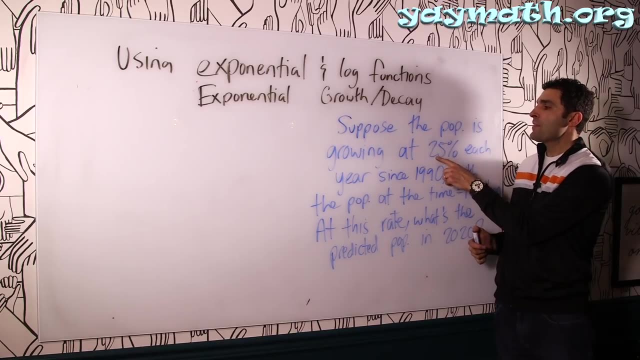 at the time, equal to 1 million. At this same rate, what would the population predicted to be in 2020.. So, basically, 30 years from there. okay, case, we'll notice that, since the population is growing at 25%, this is no. 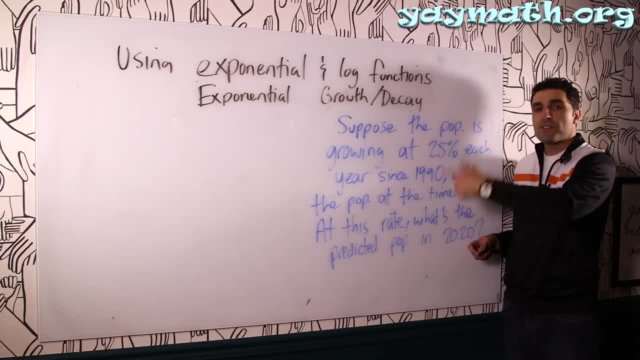 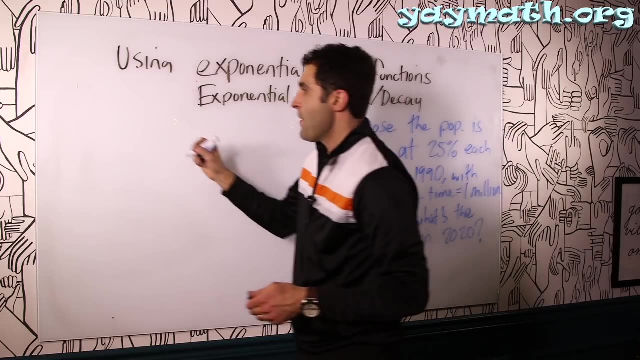 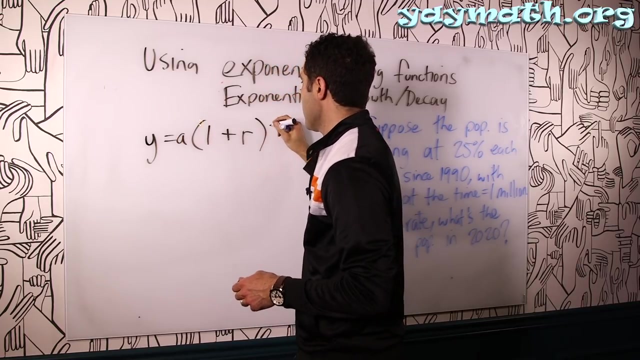 longer the exponential function, because it's not this continuous rate of growth that's naturally occurring. right, it's sort of a, it's an artificial 25% every time. okay, so we're going to use the non exponential function and we're going to go back to this guy. y equals a, 1 in this case, plus R to the T. okay, so let's find. 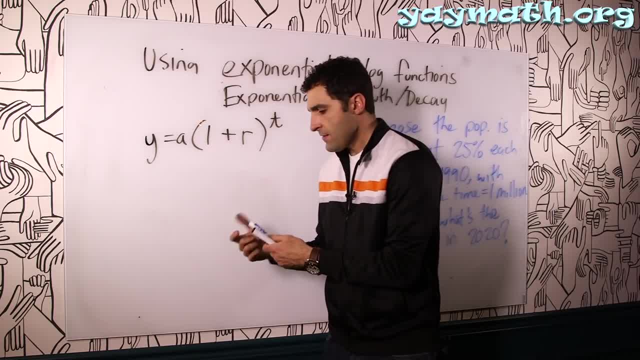 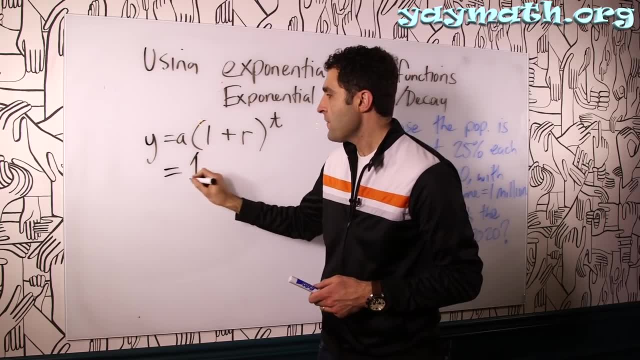 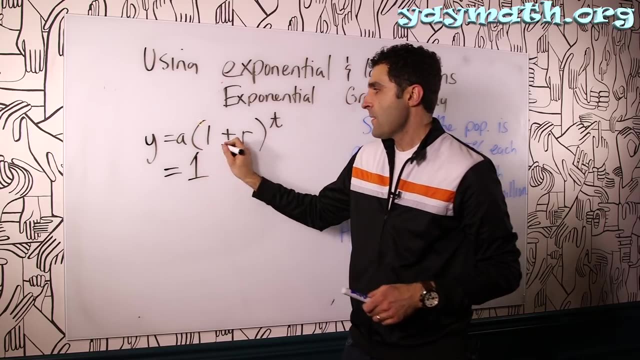 out in this case. we know the starting amount is 1 million. that's the starting amount that goes there, but you know what? can just call it 1 and just assume that this calculation now deals in millions. okay, so this is 1 million. make a guess. 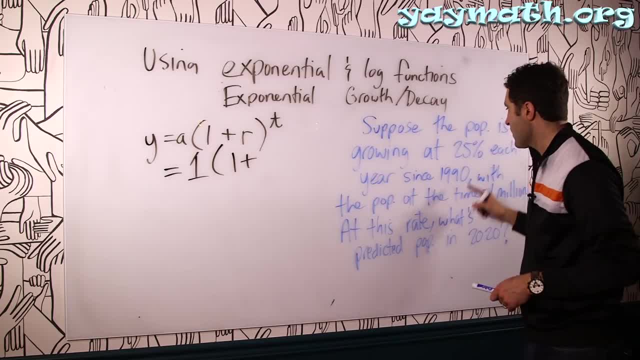 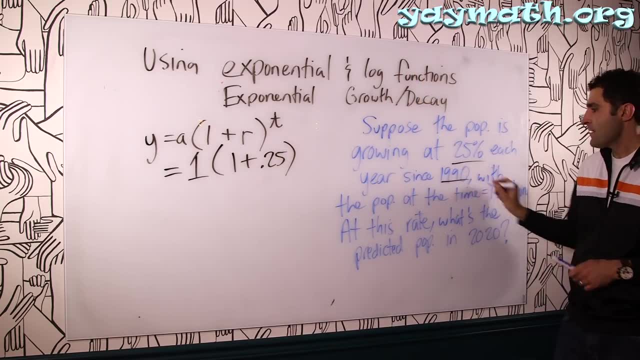 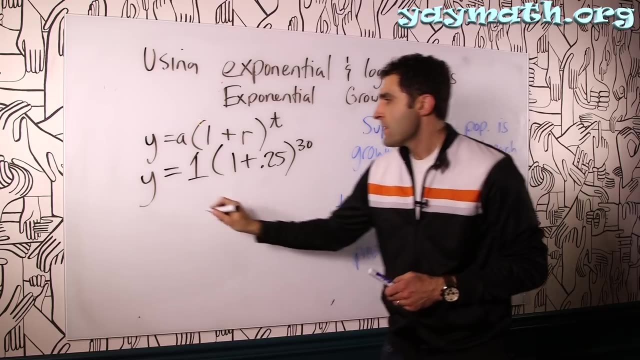 our lives a bit simpler: 1 plus the rate, in this case 25%, will be 0.25. and then we have amount of time from 1990 to 2020, that's 30 years, and we're solving for the population there. so this becomes 1 times 1.25 to the 30. all right, it's. 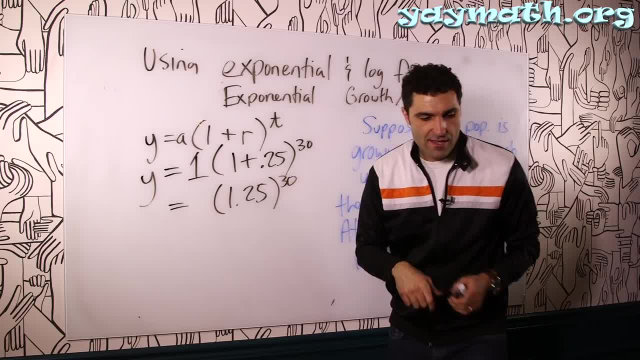 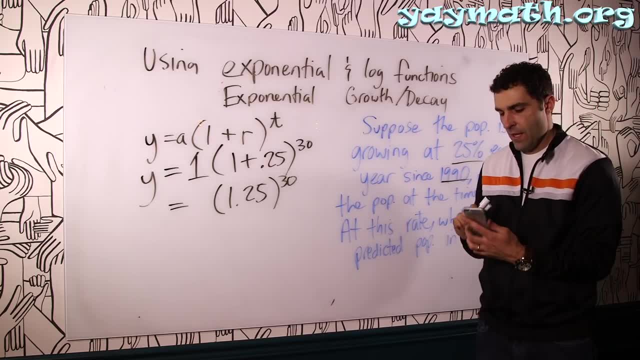 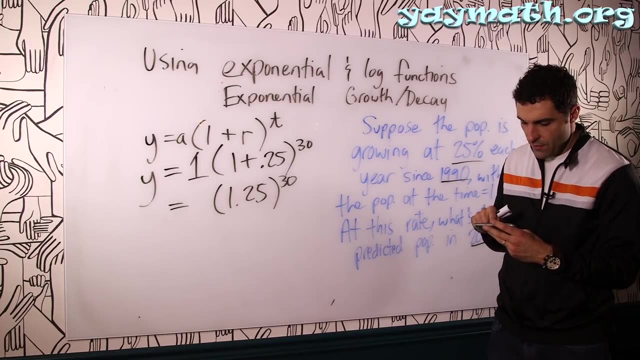 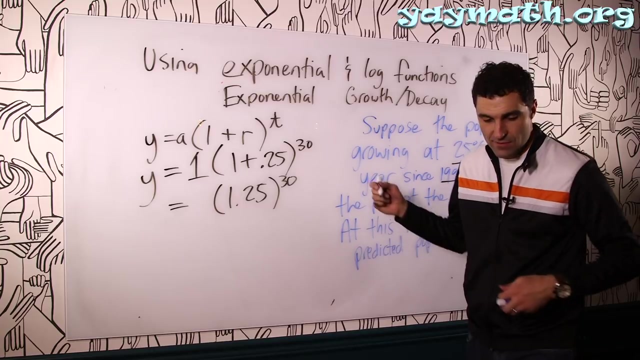 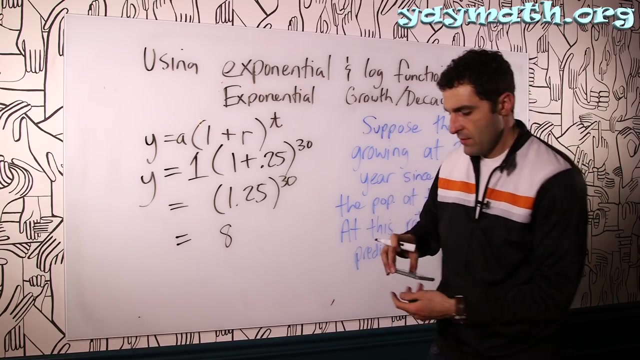 taking 1.25 times, itself 30 times, and we'll see that new population right here it is boom, okay. okay, here it goes: 1.25 to the 30- whoa, look at that, that's an explosive population. that is 8 o 7.8, then that nuts. that's 2.5 to the 30, and then that's. 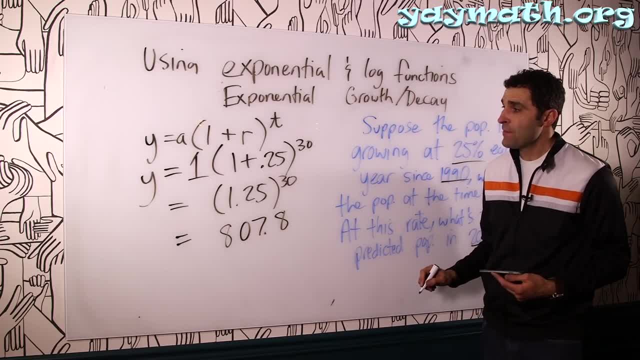 1.25 points to the 30.. okay, here we go. 1.25 to the 30.. whoa, look at that. that's an explosive population. that is 807.8. isn't that nuts? that's massive population growth. 25, that's huge. that means for every four people. 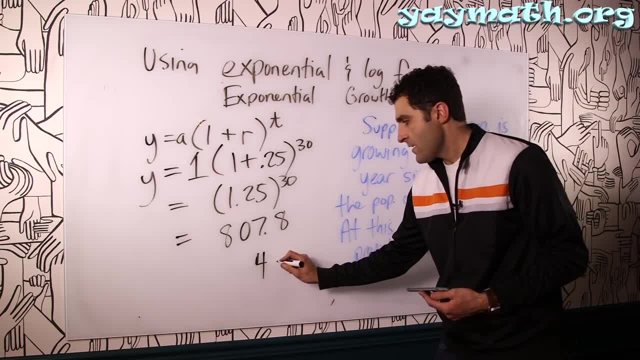 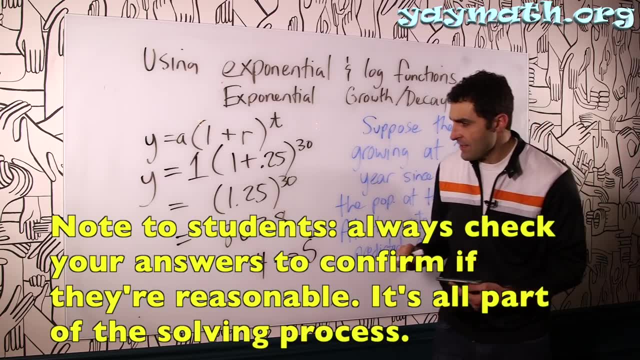 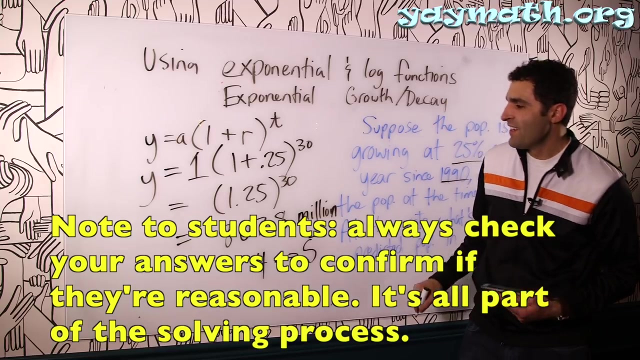 that live there. the next year, 25 more would be five a quarter of that. so one more that can't. is that right? that's incredible growth. 1.25 to the 30, yeah, yeah. so that would mean in 30 years, whatever city that is, or country for that matter- is expected to have a population of 807 million.